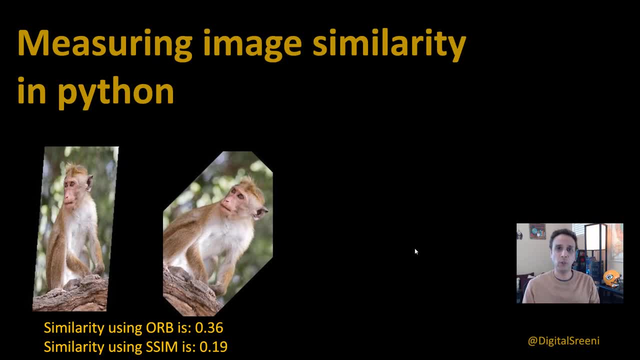 the question is: how do we quantify? is this image like 34%, or what value can we give to consistently compare a couple of images? okay, for that I'm gonna use sift or orb and SSIM metrics. okay, if you know what they are, then obviously go. 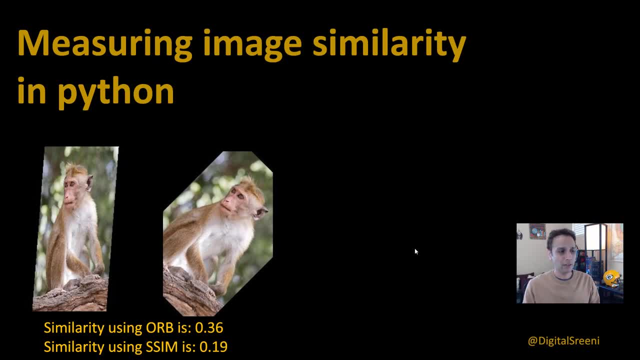 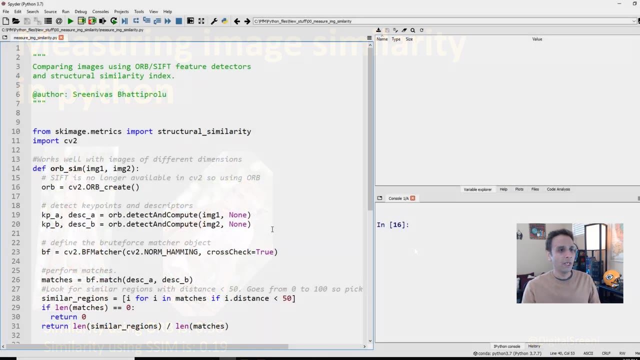 ahead and watch other videos of mine, but if you really would like to learn a bit more about how are we quickly implementing this with a few lines of code, just go ahead and watch this video. I promise to not make this very long, okay, so it's worth your time. so let's jump into the code and get to it, okay, so here. 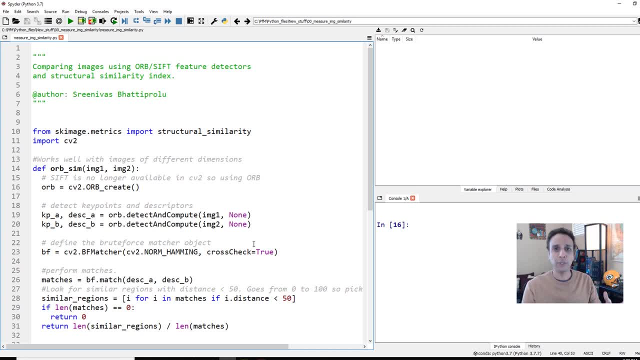 we have these few lines again. as usual, I'm going to share this file with you. look for the description. you know you'll find the github link and you can download this and all other you know code of mine that I've generated as part of this video tutorial. so please do. 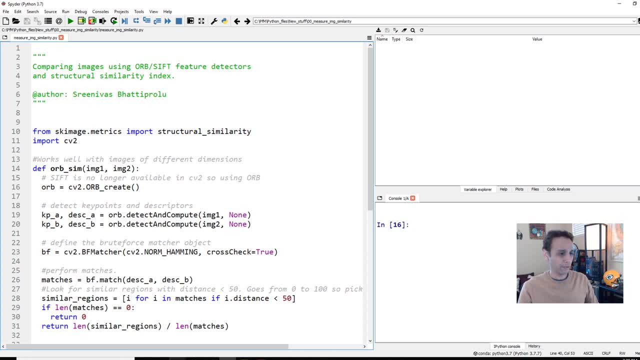 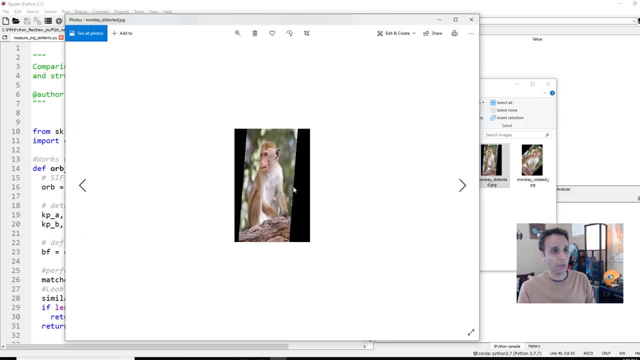 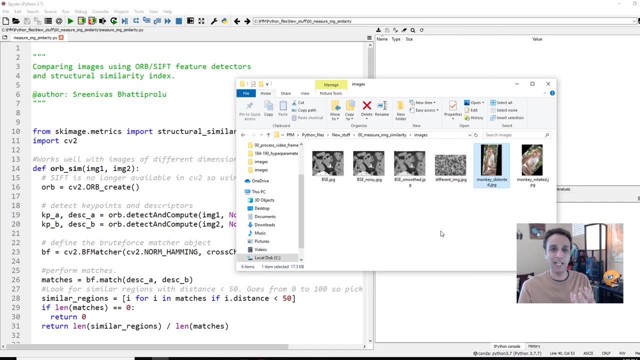 subscribe, okay, okay. so here let's define the problem. I have a couple of images, okay, the same images you saw on the opening screen. I have, for example, this warped monkey and then this rotated monkey images, and if I want to compare these two, like what is the quantitative value, and later on again, I'll also 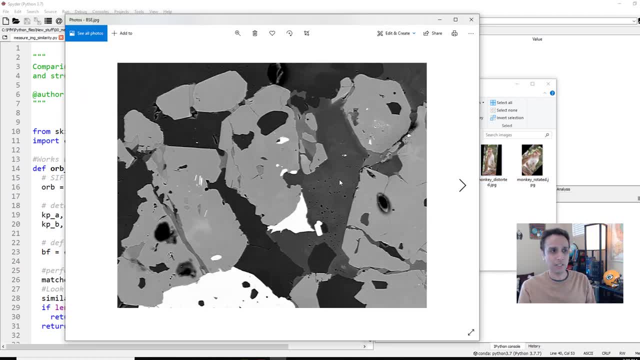 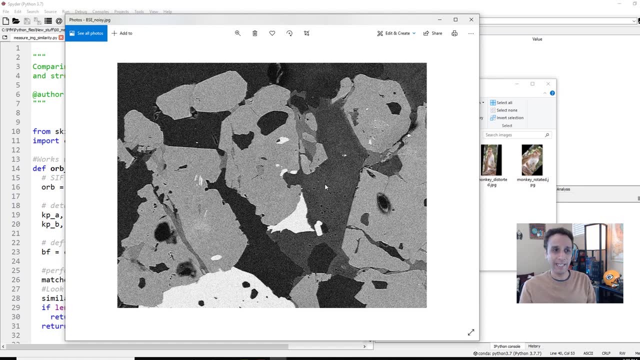 open a few other images, like scientific images. I have a very nice scanning electron microscope image, here backscattered image and here is artificially added noise, but pretty much the same image. so what type of values do we expect using exactly the same approach? right now we can say, okay, this. 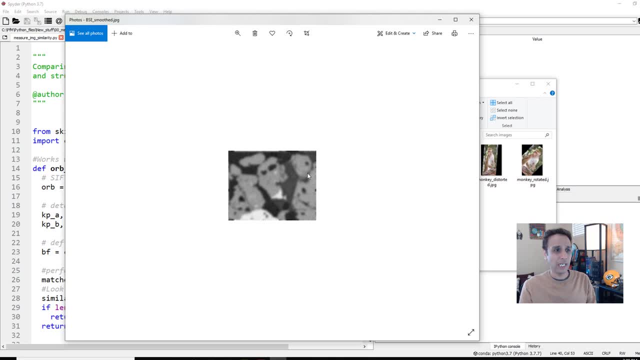 is what percentage of these images similar? and, of course, I have another image that's completely resized and blurred. now we'll see. you know what type of values can we actually expect? okay, so this is, this is the goal of my research. okay, so this is this is the goal of my research. 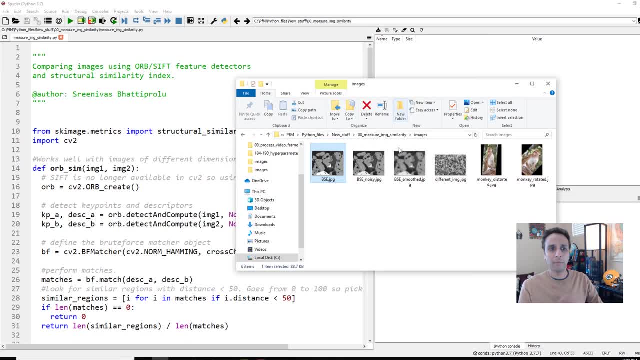 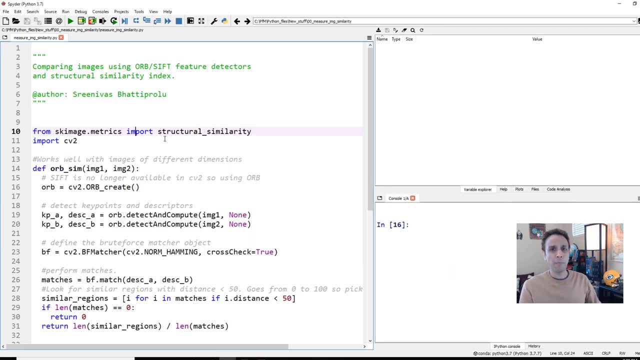 And in fact, I also have another image that's completely different compared to everything else. So again, so this is the plan. Okay, so one of the metrics. there are many metrics that claim to compare these. Well, I shouldn't say claim, but that does you know. try to compare features or different images. 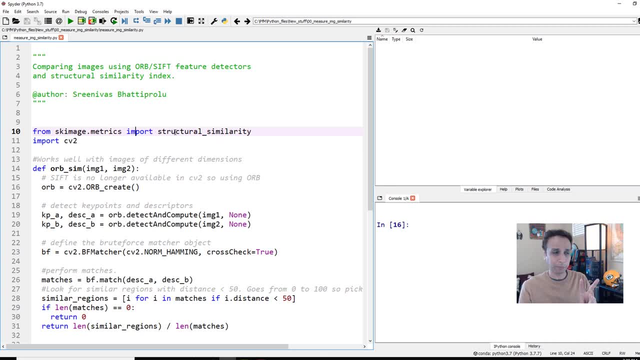 But the ones I totally rely on are two. One is structural similarity. This is part of scikit-image metrics. Go ahead and look at the documentation Again. this is not a tutorial about structural similarity, so we're not going to cover the- you know, math side of it. 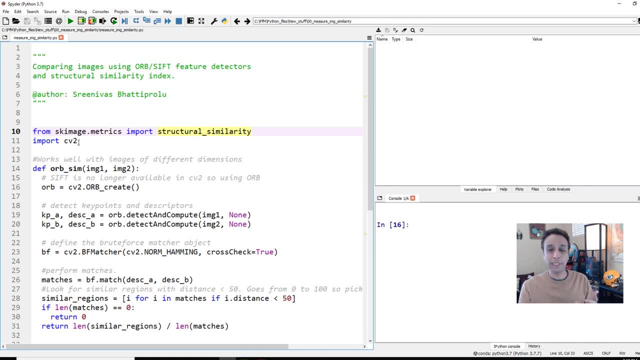 But this is one of the ones that I'm going to use, And the other one is in OpenCV. we have an ARB keypoint descriptor. It used to be SIFT. I mean, I used to use SIFT quite a bit, but they pulled it in OpenCV too. 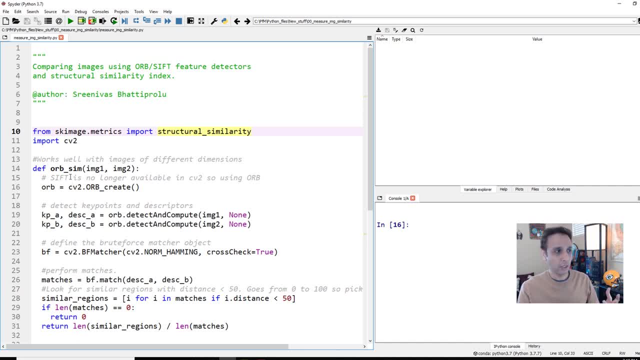 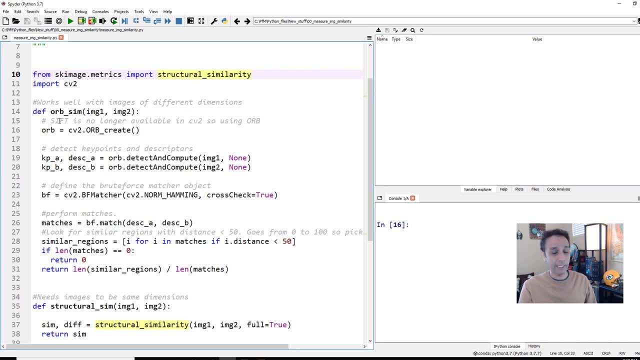 You don't have it, you know available anymore, I guess, because the original authors don't want it to give it away. You can get it for free, for whatever reason, not blaming them, but it's not available anymore, okay. 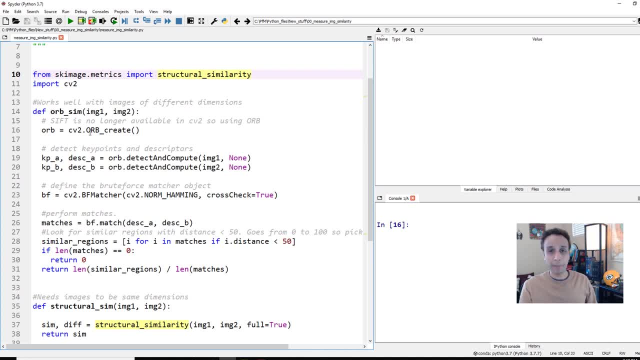 So what we're going to do is ARB, O-R-B, which is a keypoint, you know- locator and descriptor, right? I mean, it tells us: hey, these points are similar in these two images and they tell us exactly where the locations are and also describes them. 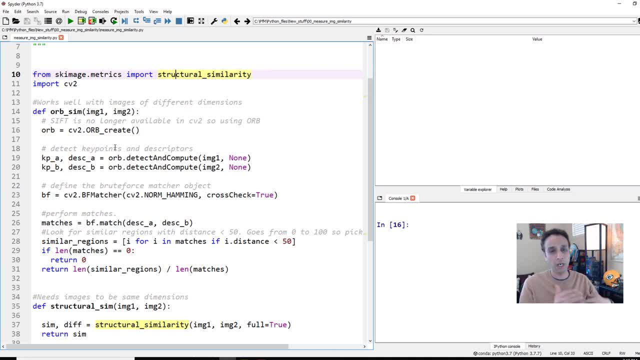 And please watch my video on this specific topic, where I talked about homography and other stuff. But let's get back here. So ARB is going to. It gives us the keypoints and describes them. It also describes them. So I create a function right here so I can apply it on multiple images right later on. 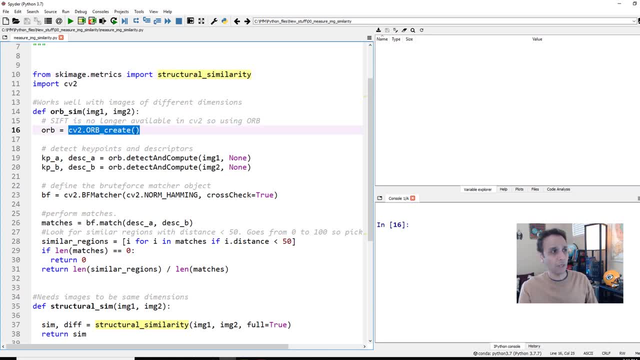 So all it's doing is from OpenCV, we are creating an object for ARB and I'm going to apply that and detect and compute on my image number one, which I'm going to supply pretty soon, and image number two, right. 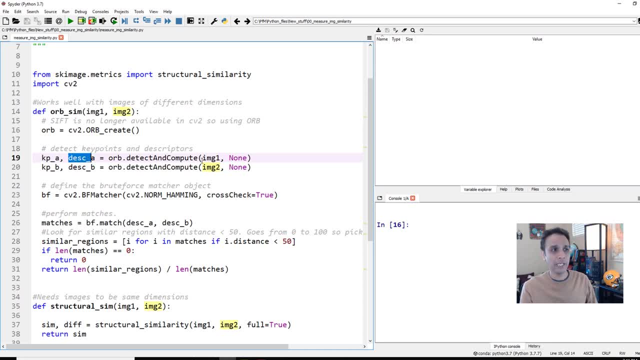 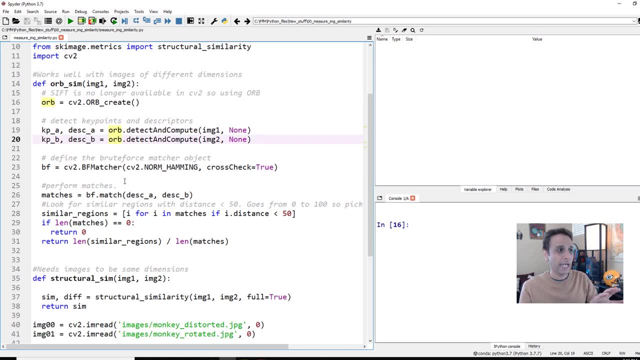 So I have keypoints and descriptors corresponding to each image. Very simple, This simple. And then, once I have the keypoints and descriptors, now I am going to perform a brute force matcher. okay, Again, if none of these make sense, you really have to go back and read a bit of documentation about brute force matching. 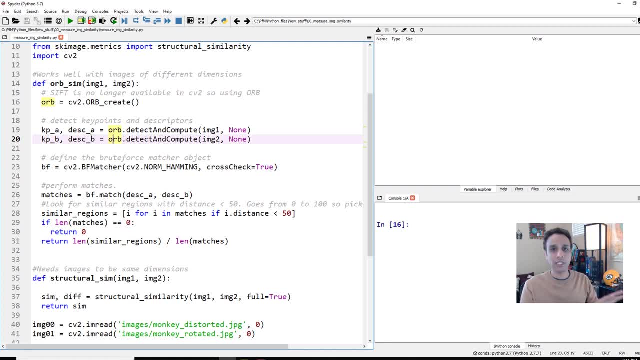 and keypoint descriptors. But to use this, it's very simple, okay, So now we are defining a brute force matcher object. now, okay, Remember, we defined an ARB object and we applied that onto our images. Now I'm going to define a brute force. 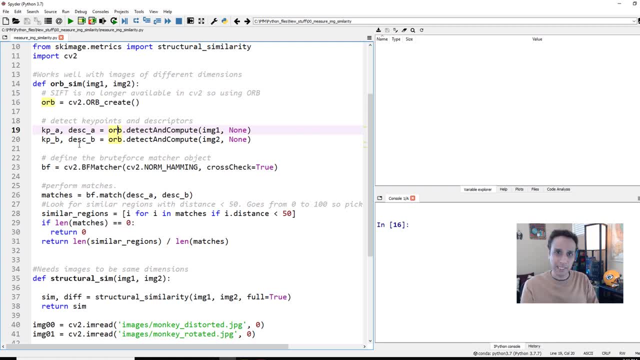 A brute force matcher and then I'm going to do something with this keypoint in a second. okay, So the brute force matcher is going to be applied onto our descriptor A and descriptor B, Descriptor A and descriptor B- right, I'm not just looking at keypoints. 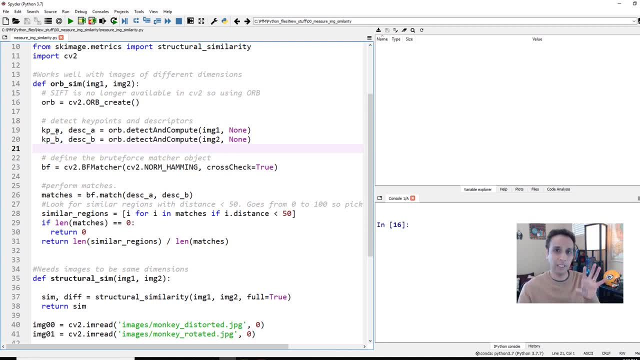 I don't care about keypoints, because now I want to see if the images are similar. So I'm only looking at the descriptors corresponding to those keypoints, okay, And I'm going to match them. So that's what brute force matcher is And what it gives you is. 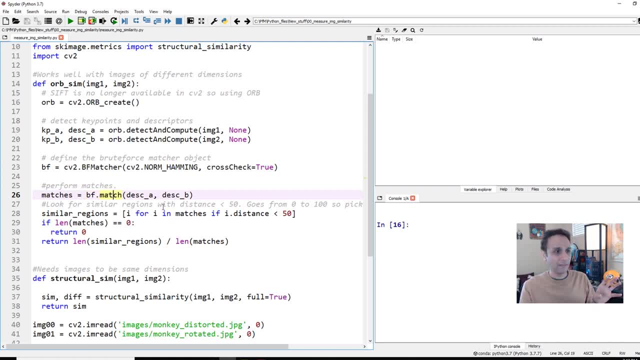 It's almost like a similarity numbers And if the number is Basically, the range goes from 0 to 100, okay, I believe 0 is perfect match and 100 is not similar in these matches. So very good matches have lower values. 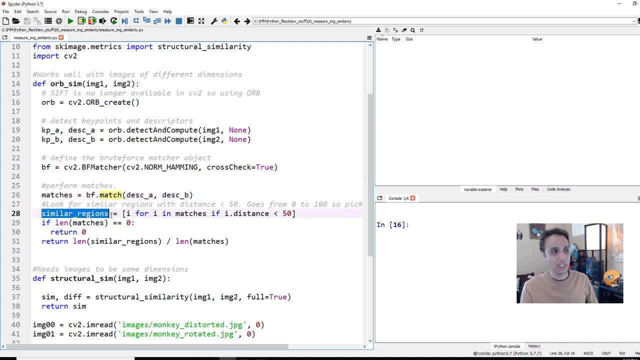 So what I'm going to do is now I'm going to extract similar regions where I set a threshold of what I call acceptable similarity. So in this case, I just say, okay, show me all the matches, Where are the differences? So the distance within my matchdistance, okay, is less than 50.. 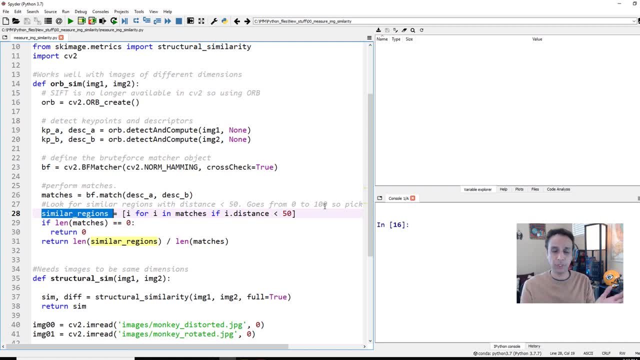 It's just 50 because it's halfway between 0 to 100.. It's up to you what you want to choose, And that's it. After that, to quantify that into a similarity value, all I'm trying to do here is look at how many of these regions follow this criteria of distance less than 50.. 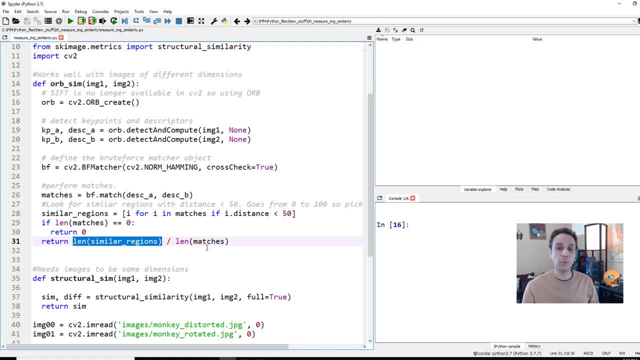 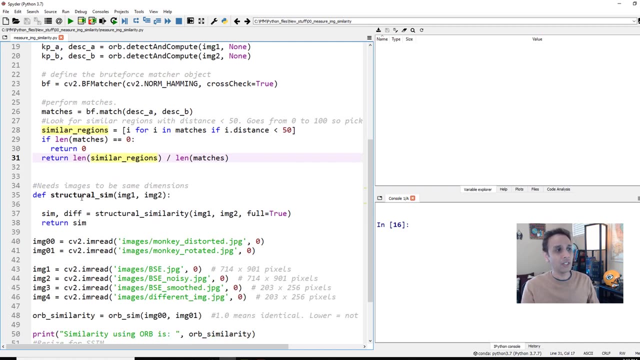 Divide that by the total number of matches, right, If I have only 20 of them below this threshold of 50 and i have total 100 of these, then i have a 20 match between these two. that's it. that's, that's pretty much it. so this is using orb descriptor, okay, and then, uh, structural. 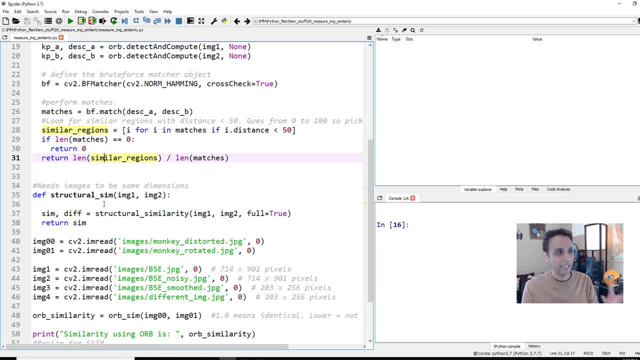 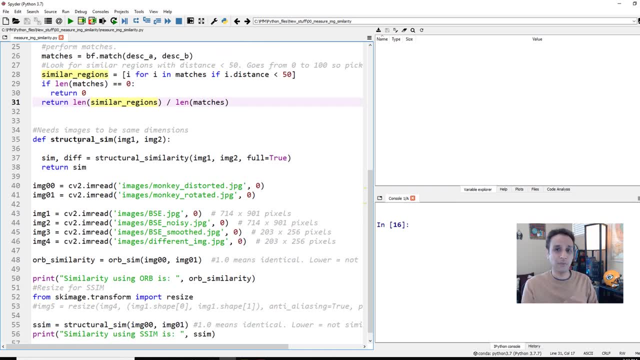 structural similarity is going to give you a number. okay, again, look at the documentation for structure structural similarity. but uh, the only thing with this is both images need to be of same dimensions, so you have to resize it if you're trying to compare images that are of different. 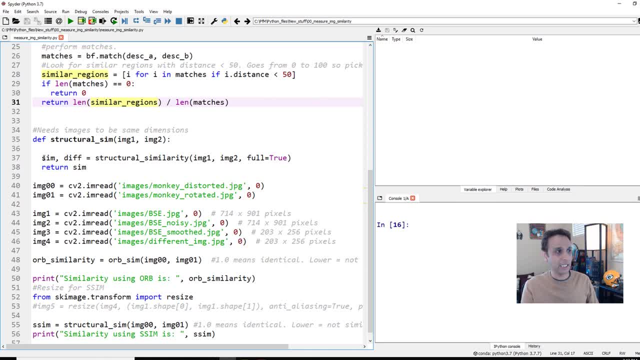 dimensions, but otherwise structural similarity. again, it's uh returning your similarity and difference and structural similarity. again, very simple, just your reference image or image one and image two and uh, similarity index. okay, uh, right there. so, uh, once we we just established what we are trying to do. now let's define two images. these: 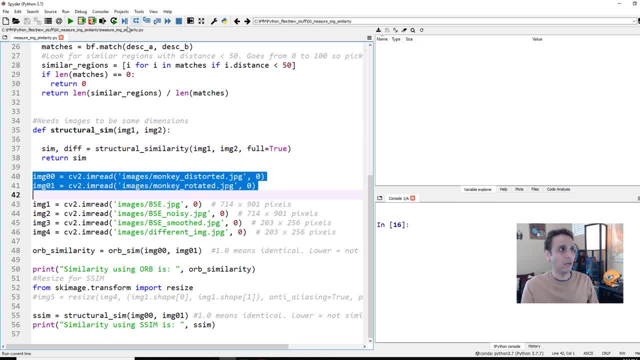 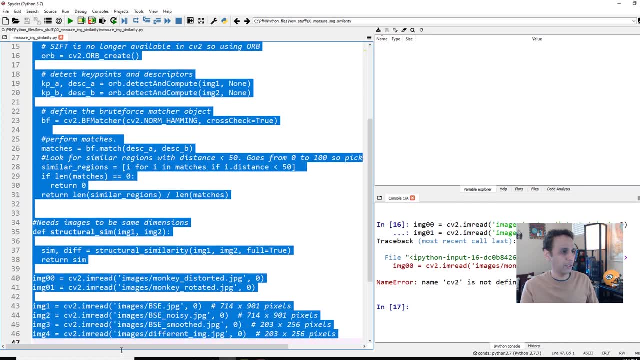 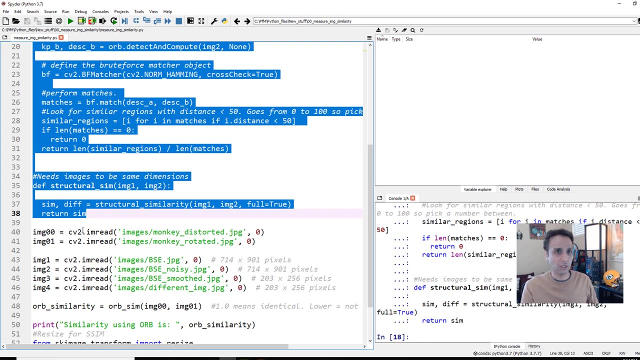 two images are the monkey distorted and rotated. so all i'm doing is just go ahead and reading. sorry, i should run this entire entire code. okay, all the way up to this. so now that we define our functions, we just need to apply the functions onto our images. so we need to read: 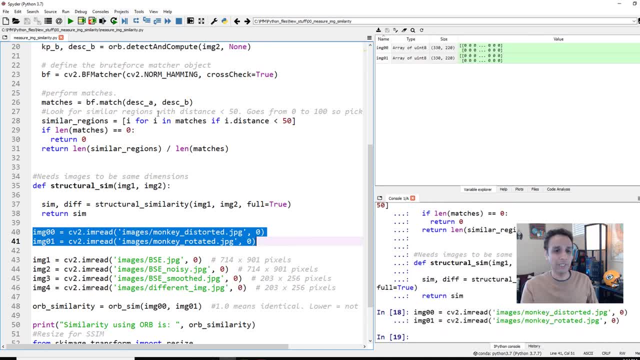 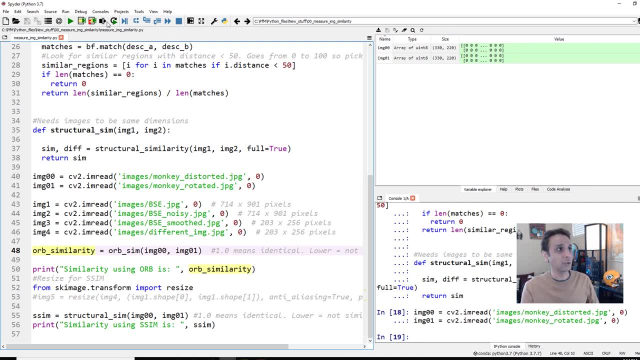 these two images. these are the monkey images, so let's start with them, and they both are same size. and now, orb. similarity is: we just defined the function. i just need to provide these two images as inputs and let's go ahead and print out what it tells us. so it's saying that the orb 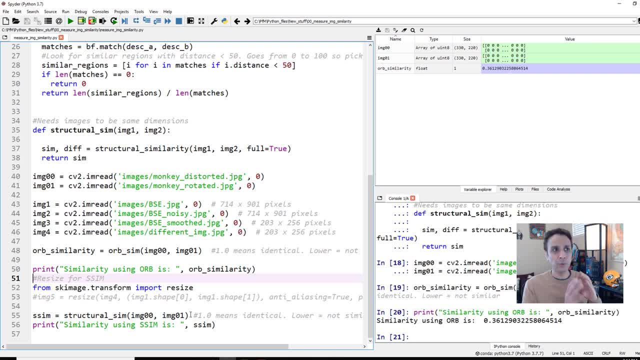 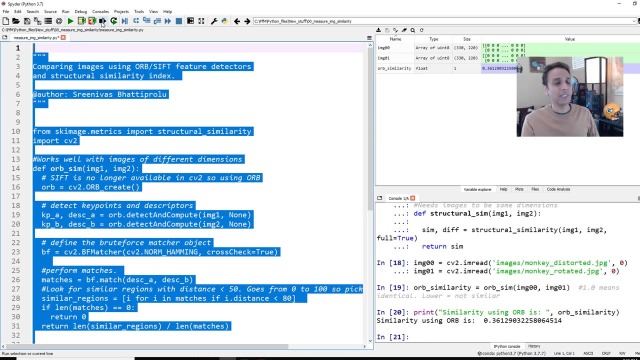 0.36. you can think of this as 36 percent. if you just not change this 50. by the way, if i change this to, i don't know, 80, for example, then let's run everything up to this point, right? then obviously the value is going to go up, right? so now my similarity is 99. 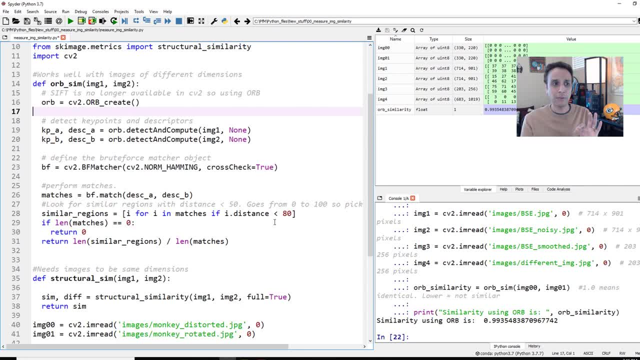 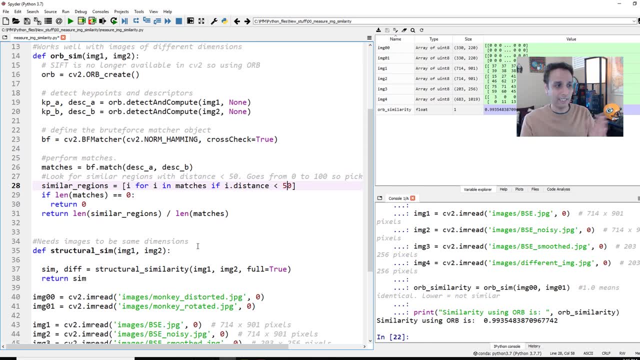 between these two images. so now it's. it's. it comes down to you what your application is, what you think is the right cutoff value is here. all i'm showing you is how to set this, and it comes down to you, you know, defining your your specific threshold there. so let's get back to 50. 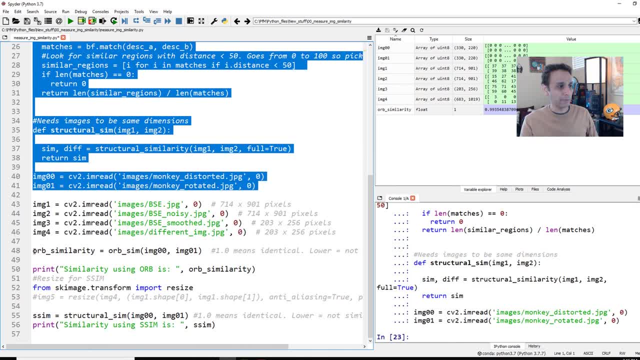 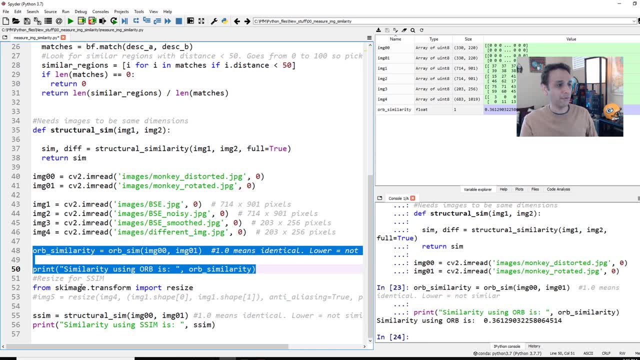 that's a comfortable point for me. and we looked at orb similarity. let's do this one more time, okay. and then, after this, let's look at structural similarity. okay, 36 percent now structural similarity. it's just, uh, uh. let's not resize because these images are of same size in this case. 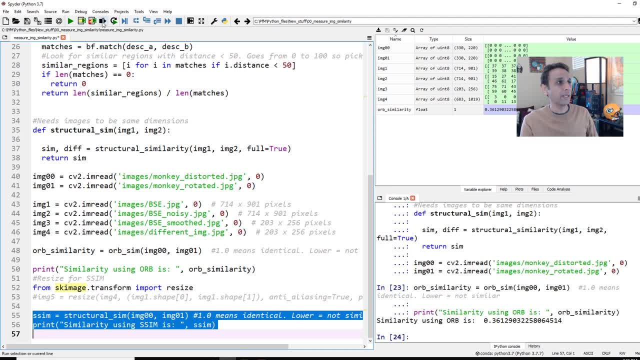 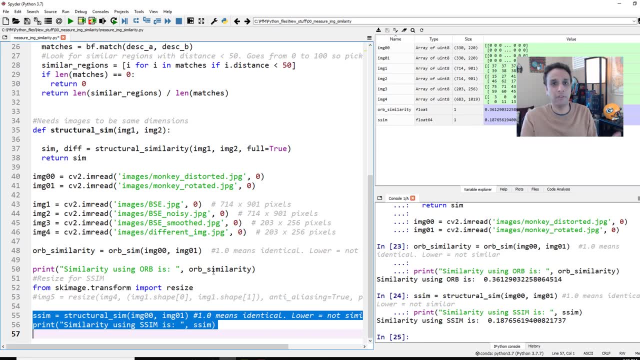 structural similarity. uh, again, we already imported the library, so it's giving me 0.187. okay, of course it's not going to be same as orb. this is a completely different process, but now you know at least a couple of ways to check this similarity. let's go ahead and run these. uh, all of these load, all of these images and 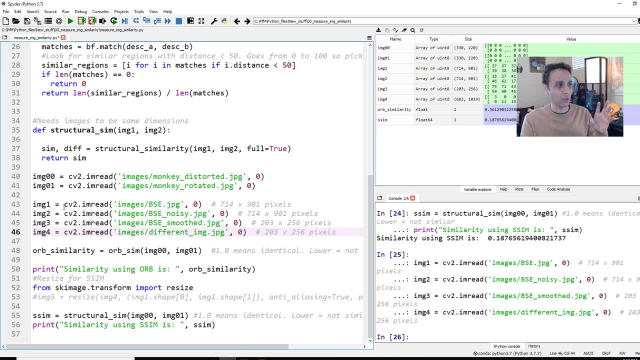 these are the ones i just showed you, right, the noisy uh. so image one versus. so let's go ahead and do image one versus image one, same image one. so let's go ahead and do image one versus image one same image. are they similar? obviously they should be. if you do that, your orb similarity is one. 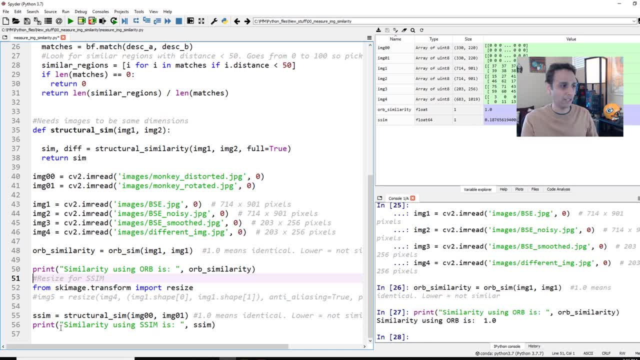 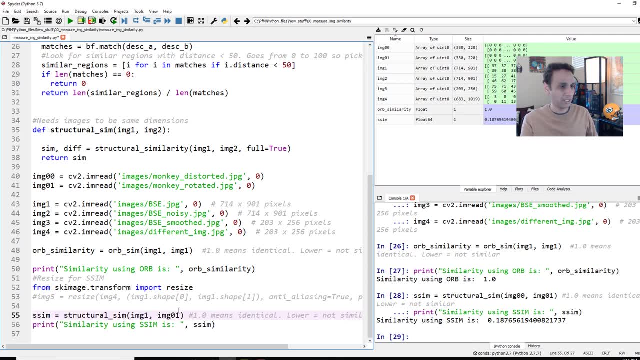 that means hundred percent. okay, now it gives you an idea of what the reference is, and let's also look at structural similarity, which should be: uh, oh, sorry, i didn't change my image number, so let's go ahead and do image one and image one, and structural similarity should be: 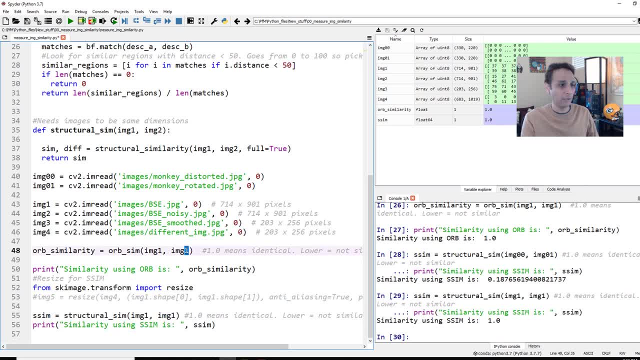 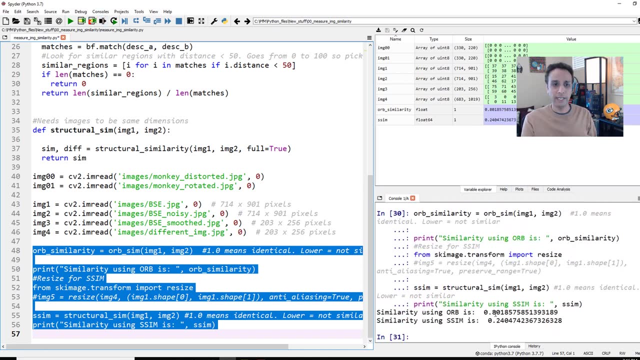 also one. okay, because we are doing exactly the same image now. uh, the same image versus the noisy image, okay, so now we are just doing this. let's run all these lines. so, um, for orb, i'm getting 80, and uh, ssim, i keep calling 80, a value of 0.8. and for structural similarity, i'm getting a. 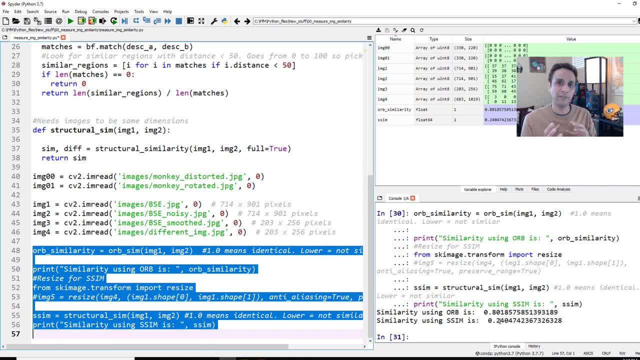 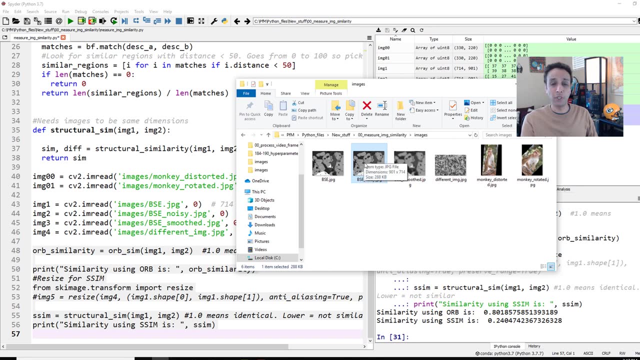 value of 0.24. that kind of gives you an idea of what the range is. you know in general. so structural similarity. it completely went down from one to 0.24 and the only difference between these two images is this: one has about five sigma noise. that's pretty much it. now let's compare the smooth to one, which is image number. 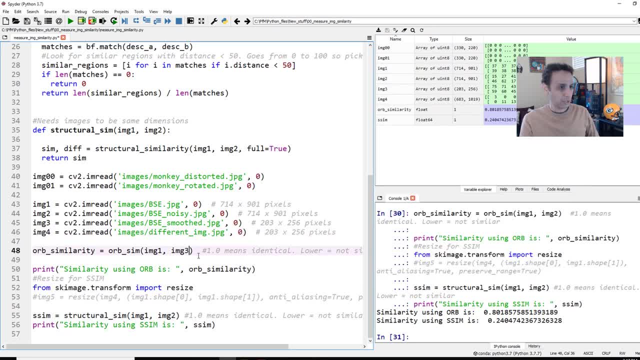 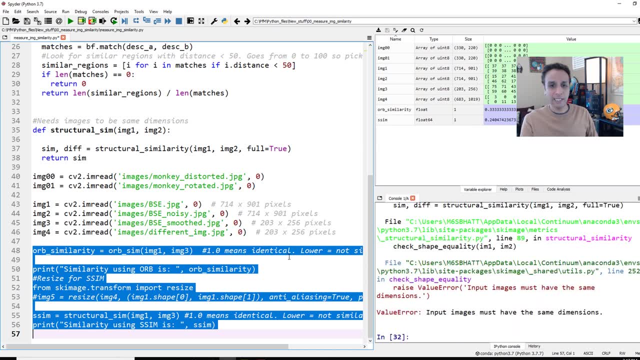 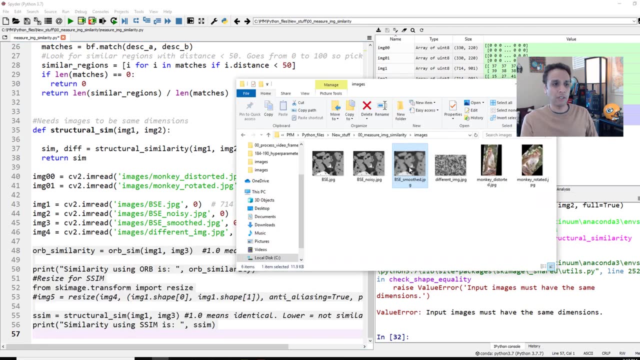 three. i believe image one versus image three. okay, so let's do a couple more and then i think you'll have enough uh information. so let's run these again and uh, it says yeah. as you can see, input images must have same dimensions, because my blurred image is much smaller than uh. 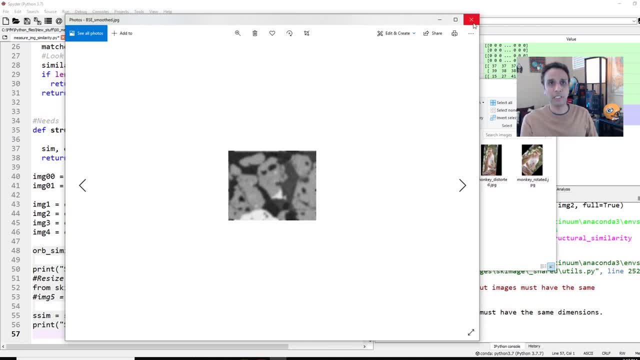 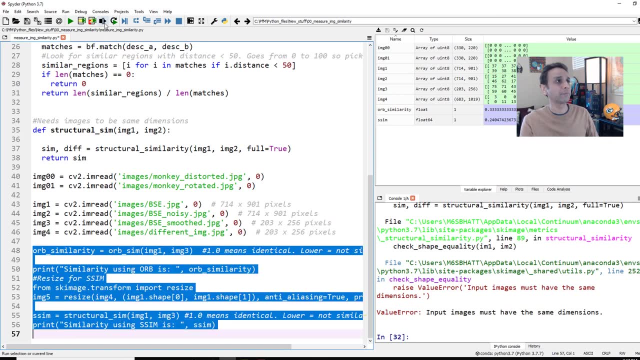 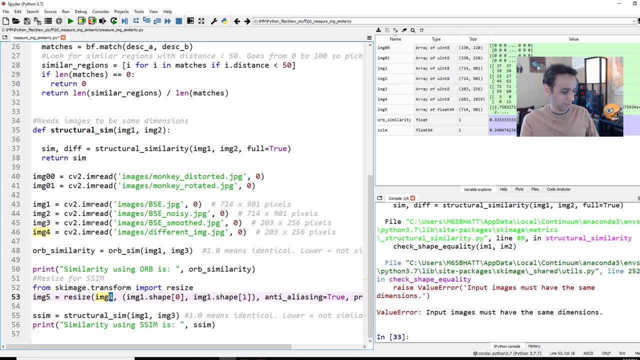 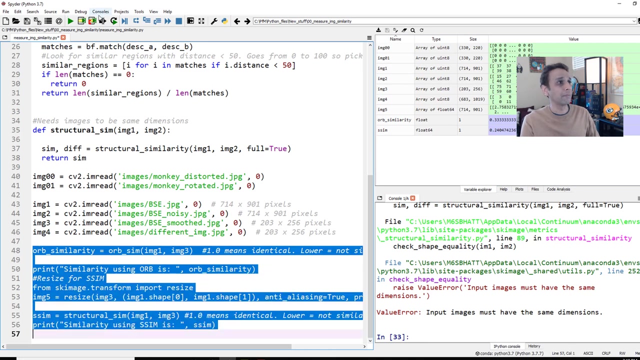 the other images, as you can see, and the edges are crappy and everything. okay, so now let's go ahead and resize this image and let's run this one more time. um, i thought i'm resizing it, uh, image. sorry. resize image three. i was resizing image four. okay, uh, third time is a charm, so let's do that. 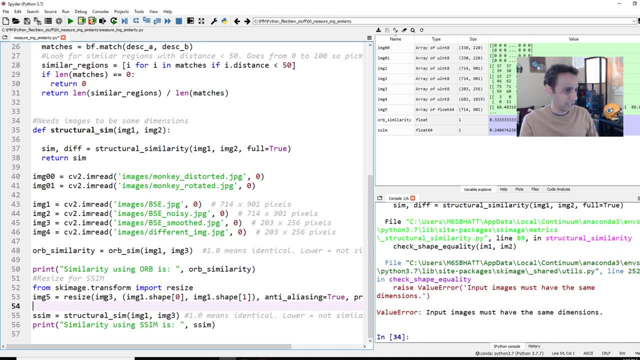 okay, i think i'm- uh, i have to focus here. resize, uh uh, image three and uh, oh, my god, too many things to change. that's what happens when you don't write the code in an efficient way, where you have to change the same thing multiple times. 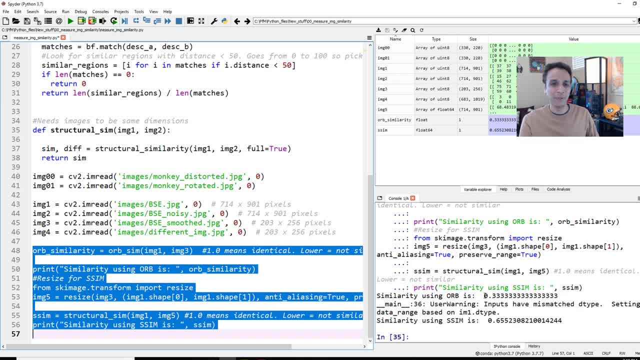 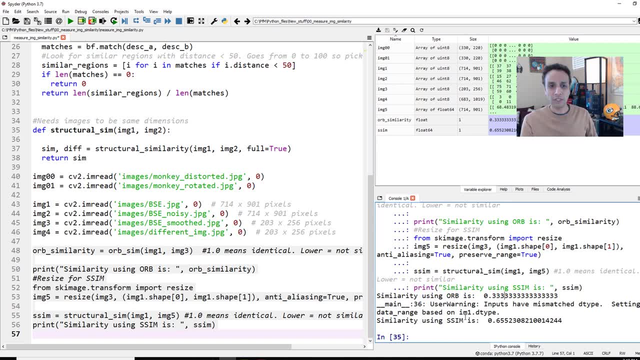 okay. so if this doesn't work out, i don't know what. okay. so there you go. so here it says: uh, similarity of orb is 30: 0.33, but then the structural similarity is 60: 0.65. so when i resize this, it's: 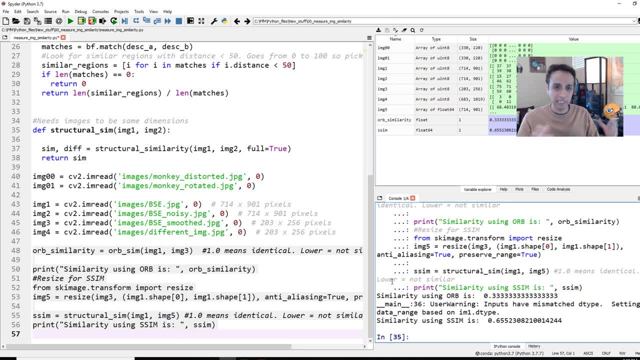 looking at the structural similarity right between these two. so once we resize, apparently it thinks uh, it, it's, it's uh similar. so i if if you're trying to follow this method, i definitely recommend using these two parameters when you're looking at structural similarity. maybe you want to take 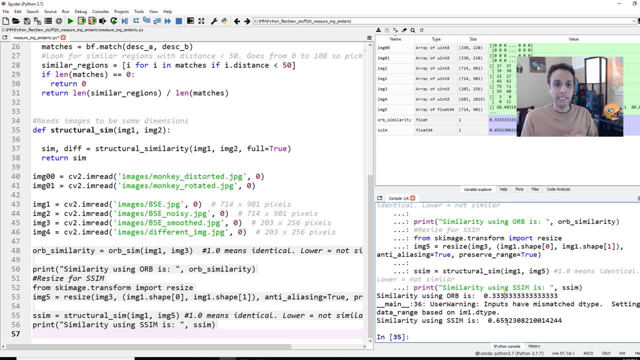 an average. maybe you want to write another function to say if orb is this and if ssim is this, then okay, i want to say that this: these are similar- or now i leave it to you how to use these two- but kind of different. they're looking at different aspects and they're giving you these. uh, um you. 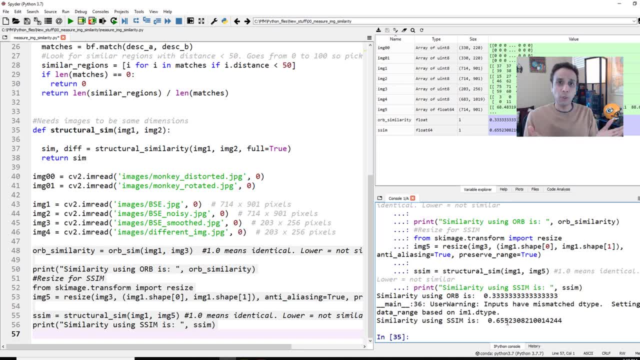 know these, these uh numbers out there, okay, so i hope i hope this answers you guys's questions that you left in under comments. so if you have any such questions, please do leave here, unless unless it's a humongous project for me, if it is relatively easy for me to explain. 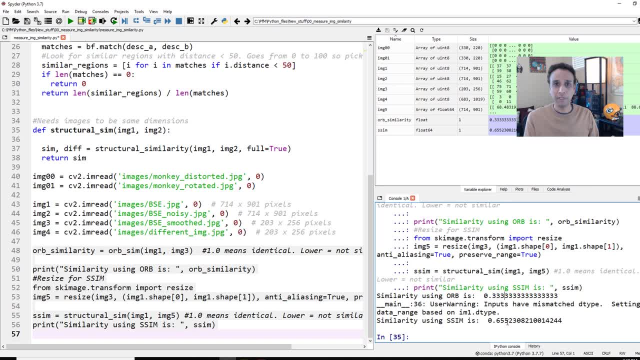 i'll record a video for you, otherwise i'll just leave like a comment or something. but please do engage, please do practice and subscribe to my channel and thank you very much, very much for watching these videos and let's meet again in the next video, talking a different topic. thank you. 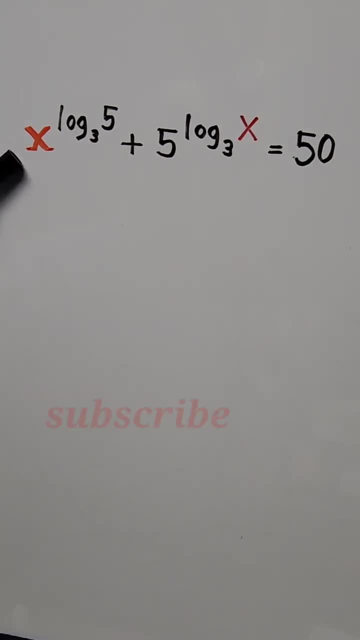 Nice logarithmic equation. Solve for the value of x. Here we use the formula a, here is x and b is 5.. So we're switching. If you notice that a, here the base becomes b, So the first term can be written as and the second term remain. 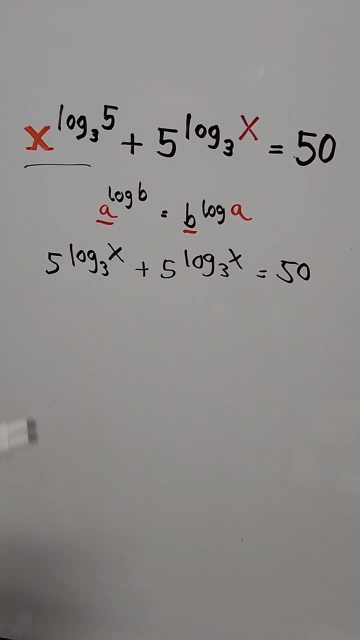 the same equals 50. So now we have two of the same thing, so we add both. So we ended up with 2 times 5. raised to log base 3 of x equals 50. Divide the whole equation by 2.. So we have here: cancel 2.. 50 over 2 equals 25.. So we now have 5 to 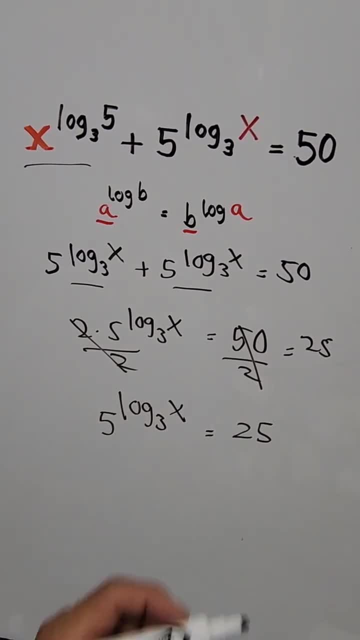 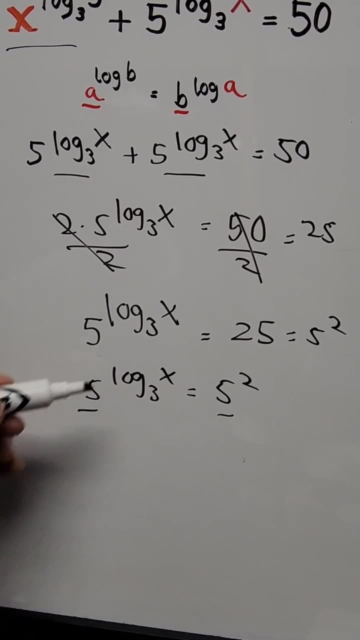 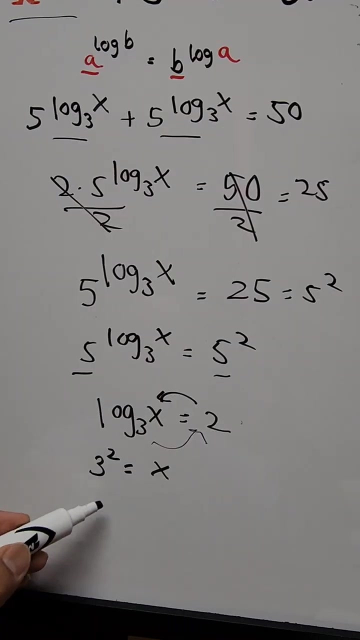 the power of log base. 3 of x equals 25, and 25 is written as 5 squared, So now we have the same base. So we now have log base. 3 of x equals 2.. So now transform the equation into its exponential form: 3 squared equals x, So x is equals 9..